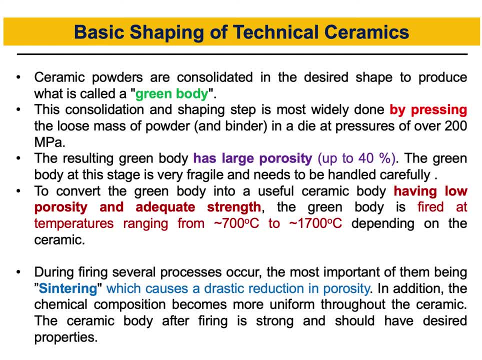 Dear students, welcome and thank you for tuning in for this video. This is the last video actually of the ceramics lecture, which is part of the material science class and the biomaterials class, and we're going to talk in this video about the basic shaping of technical ceramics, or 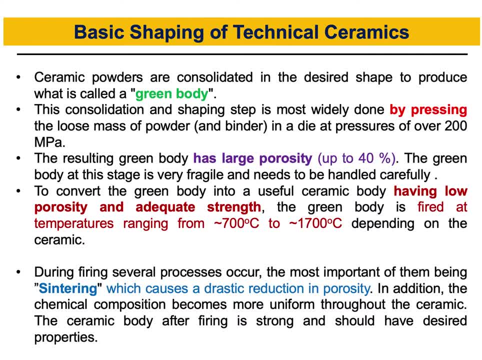 engineered ceramics or fine ceramics. that's what we call them. Remember that we discussed this before, that we are characterizing ceramics by the type of applications they're used for, So for technical or engineered ceramics. how has it been made and what are the properties of this? 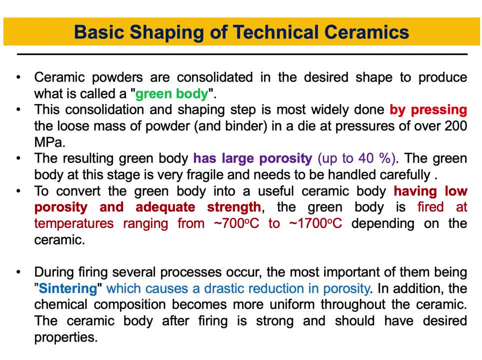 process of manufacturing and basic shaping of ceramics. So ceramic powders are consolidated in the desired shape to produce what we call a green body. A green body which means it's a soft body. So we have an object that is still soft, it's not hard, it does not have its strength ultimate. 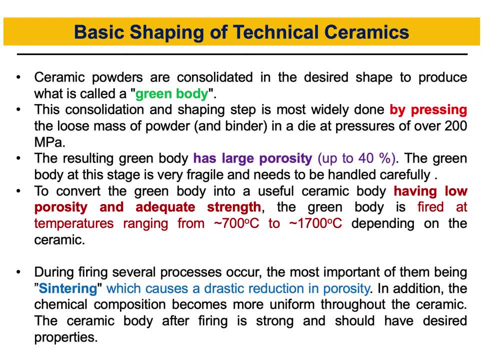 strength that we would look, we're looking for. So it's still probably. it's just like, like it's a very soft structure. Let's keep it this way. This consolidation and shaping step is most likely done by pressing, So we press the powder and the loose powder in order to create that material. 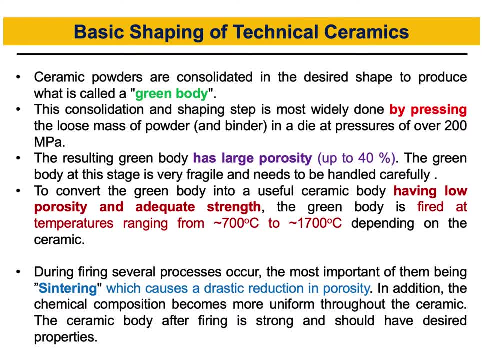 and usually we have to use a pressure of at least 200 megapascal, So it should be a lot of pressure in order to create our green body. So the resulting green body has a large porosity and it could go up to 40 percent. So we have, in any, you know, confined volume, 40. 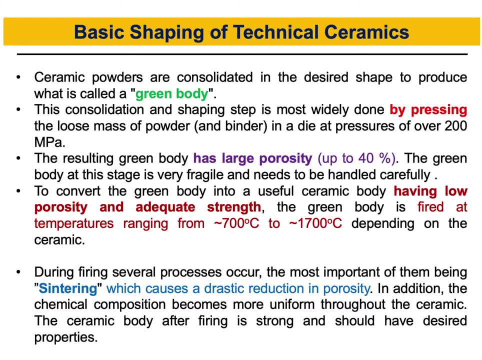 percent of that volume is void. It's porous, So we need to, you know, reduce this percentage of porosity. So the green body, it's very fragile and need to be handled carefully Because it could break. Now, to do this we have to apply temperature- you know heat- and to convert. 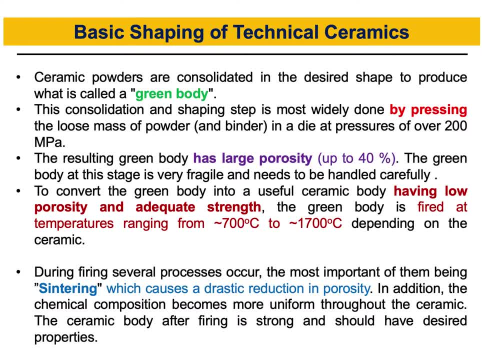 the green body into useful traffic ceramic with lower porosity and adequate strength. This is what we're looking for. We need to heat it to temperature between 700 degrees Celsius and 1700 degrees Celsius, depending on the ceramic that we are using and the material we are which we are using. 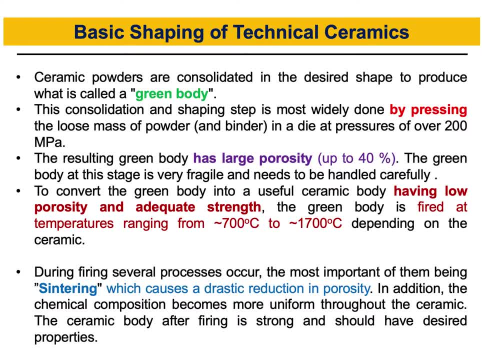 So, keep in mind, we have a green body lot, large percentage of porosity, There's a lot of void. We need to reduce porosity and we need to make it stronger. So, in order to do this, we heat it up and in heating, a lot of things happened, happens, And some of these things that happen 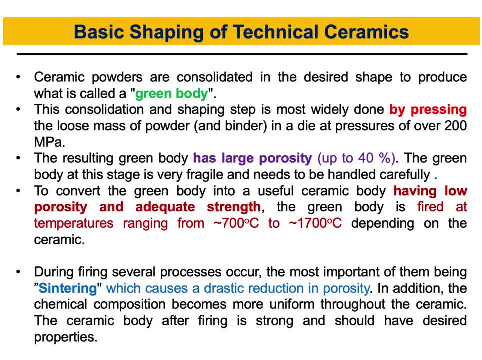 is something called centering. Centering because of the temperature, the high temperature and the firing. centering causes a drastic reduction in porosity. So we are, let's say we are- filling the voids. Now the material is filling the void by you know. 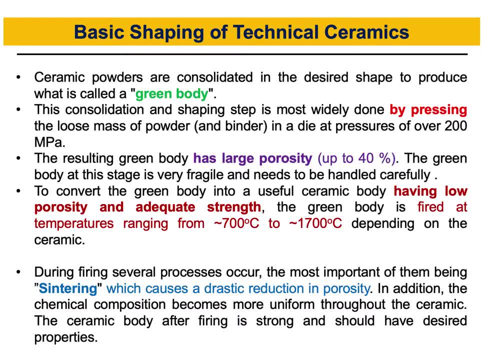 Reducing its volume, And it depends a lot of a lot of variables, But since let's keep in mind that centering is reducing, It's the way or the step where we are causing a drastic reduction in porosity. Also, because of firing and the high temperature, a lot of chemical composition becomes more uniform. 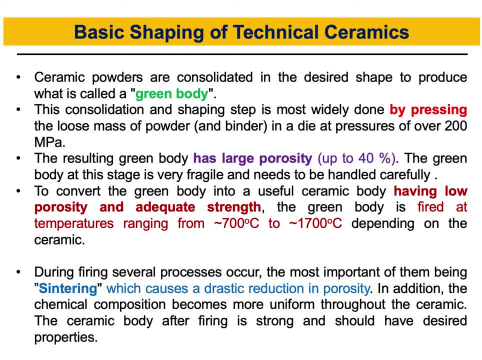 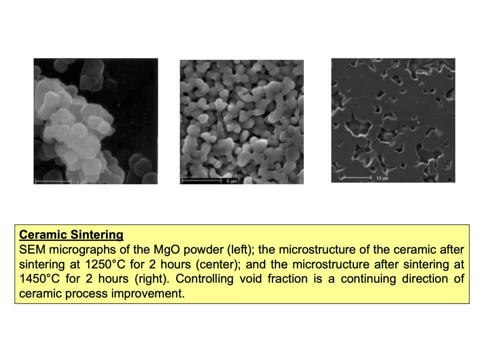 other chemical composition become more uniform- uniform throughout the ceramics- and it's becoming stronger And it will have the desired property that we are looking for. to put this in perspective, I'm going to show you this image here, and this is scanning electron microscopy images of ceramic. 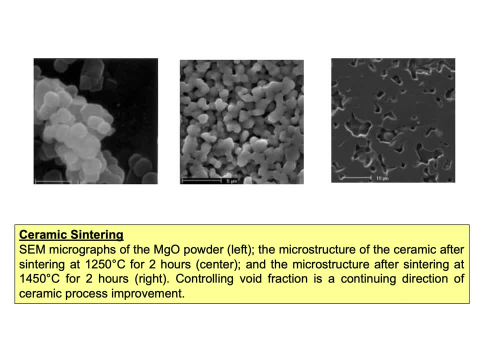 powder at different stages in the shaping process. So this is magnesium oxide powder here and it's the one to the left If you are, you know, heating it and firing it with and also, you know, at 1250 degrees Celsius for two hours, centering that center. 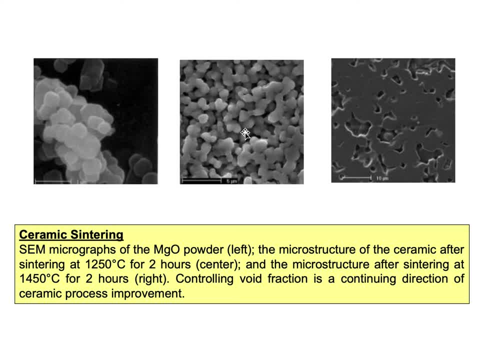 That's that process called centering. We are going to have something like this, So we have a material that is less porous. So if you look at this ceramic- this void here is air is nothing when you center it at 1250 degrees Celsius. 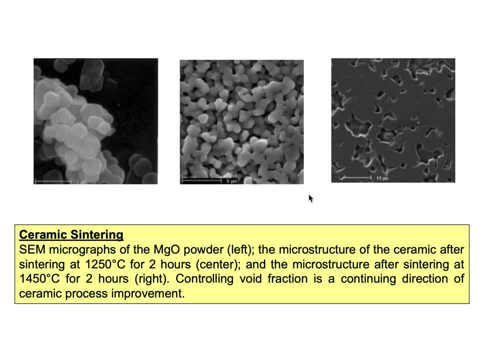 for two hours. It becomes like this: now do also do more centering For it at 1450 degrees Celsius for two hours, You're going to get the one to the right and the Microsoft author. So I think, after two hours of this stage, at 1250, 50 degrees Celsius for two hours. 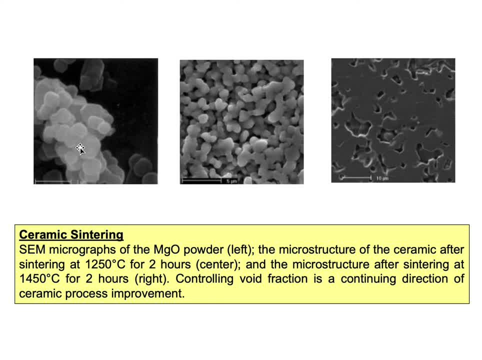 We reach this point. If you increase the temperature right and to 1450 degrees Celsius after two hours, you will reach that point. So you can see that we are we. the voids are way much less The percentage of porosity, and this is a very important application, and this affect a lot of the ceramics application that we want to use. 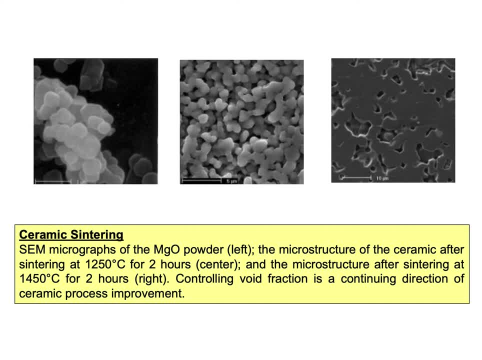 For example, in biomedical engineering. we would like to have an ultimate sweet spot of porosity, porosity for cells to attach. Let's say, if we are putting an implant bone in order to fixation inside the body and you want the cells to attach to it. 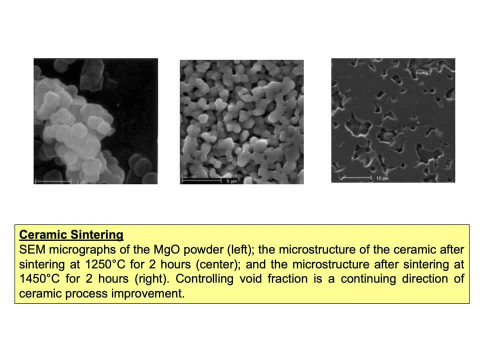 So there is Specific size, specific percentage of porosity and a specific pore size for cells to attach and to grow there to our implant. So this is how we are doing this in ceramic, how we are controlling the porosity and the pore size by centering. 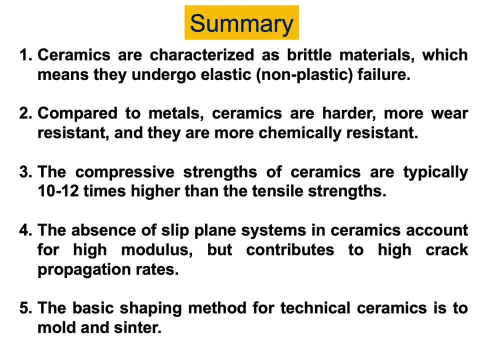 To conclude, as a summary, ceramics are characterized as a brittle material, which means they undergo Elastic failure. It's not plastic, and to show this in a little bit in a picture. So this is the: how would it look like if you have ductile fracture? 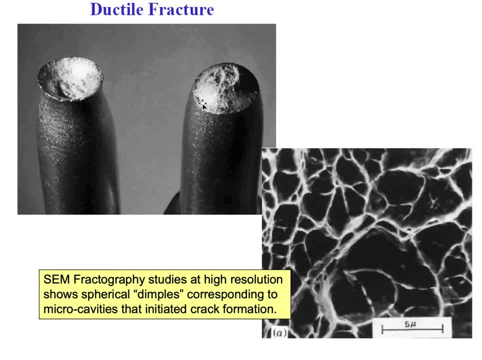 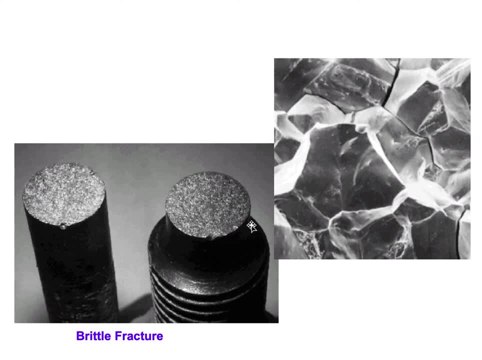 which is plastic deformation. and then you have fracture. You have this ductility of the material. if it's brittle, it will look like this. So if you look at the surface of the fracture, it's a flat, it's brittle, So we don't have any deformation or strain. that happens as in ceramics, as opposed to metals. 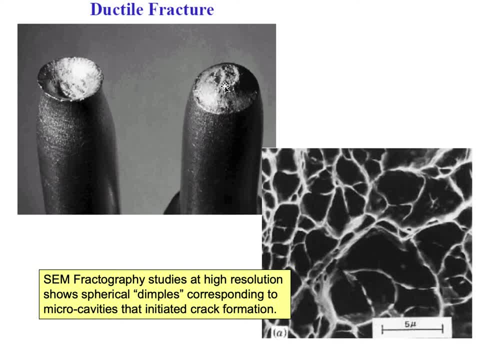 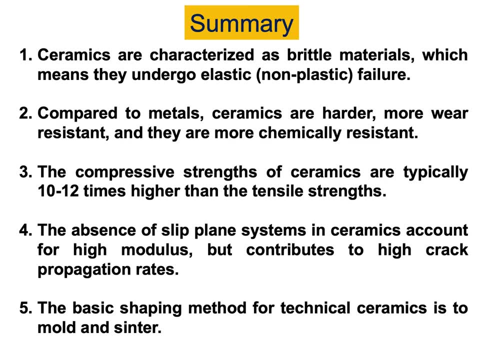 This is what happens in metals. You have this gradual plastic deformation before failure, but in the ceramics it just like this. It just frapped cracks. So this is the difference between brittle materials, which are ceramics, and ductile materials for our metals. compared to metal, ceramics are harder. 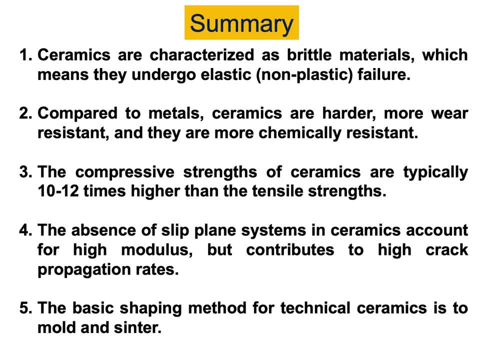 They're more wear resistance and they are more chemically resistance. They're stable and we discussed this and the reasons why this is happening. The Compressive strength of ceramics are typically 10 to 12 times higher than of the tensile strength.